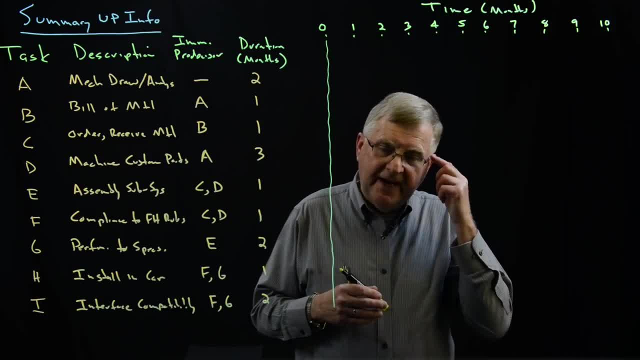 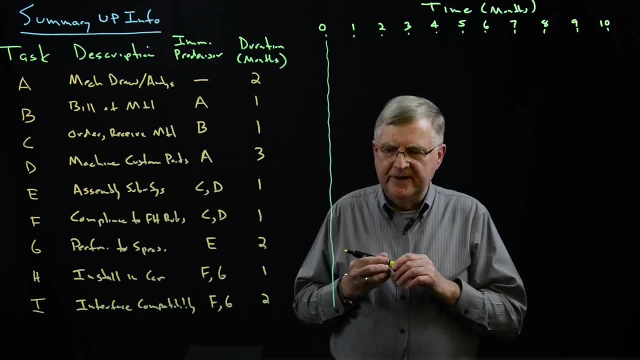 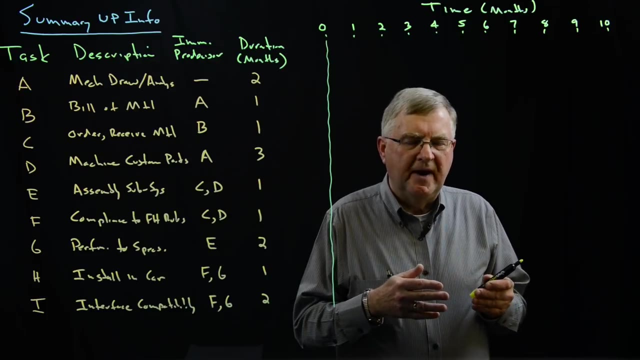 Alternative approaches. like PERT assumes that there are variations at the various times. That could be applied here also, But for this example I'm going to focus on critical path. I'm going to be looking at the design and the construction of a mechanical subsystem to be used on the race car. 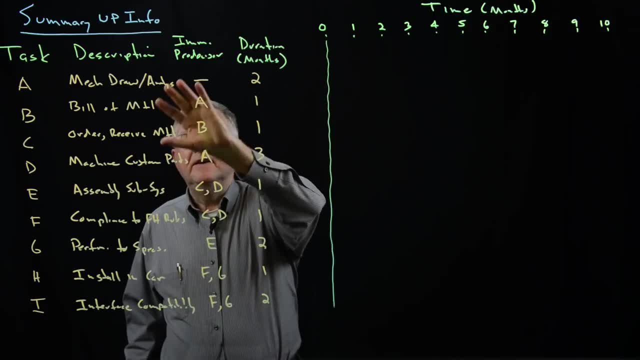 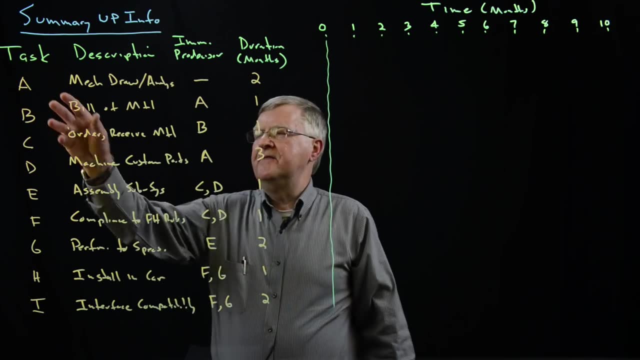 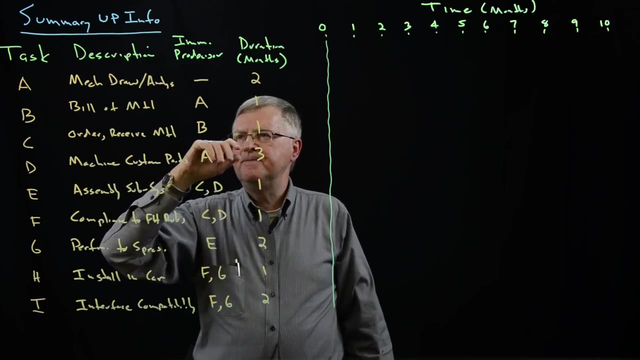 And this table here summarizes the information from the work packages that were received From the groups that are completing the tasks. I've identified the task with a letter identifier. There's a description of each task. The description indicates there's a task of mechanical drawing and engineering analysis. 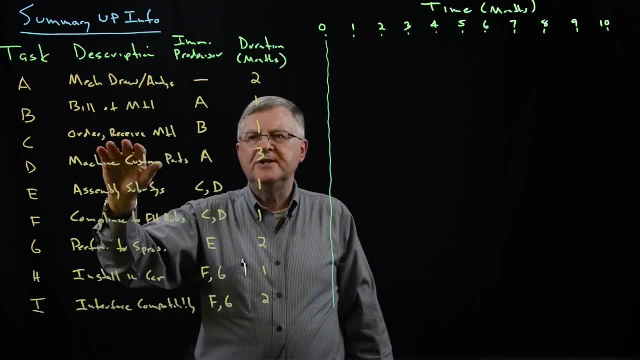 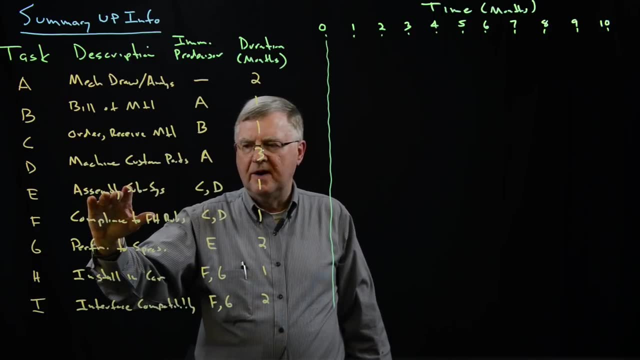 Generating the bill of material, Ordering and receiving the material, Machining custom parts, Assembling the subsystem overall. Looking to see if it's going to be a task that's going to be used on the race car- to see if the subsystem complies with formula hybrid rules. 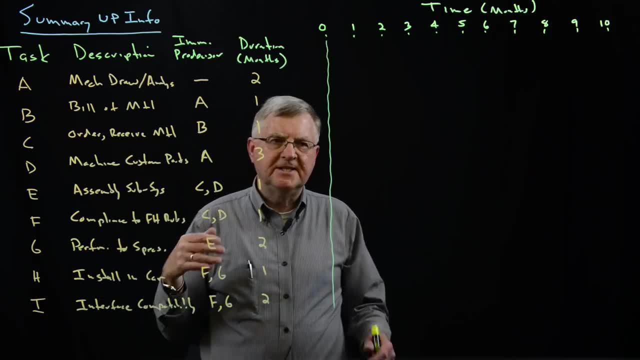 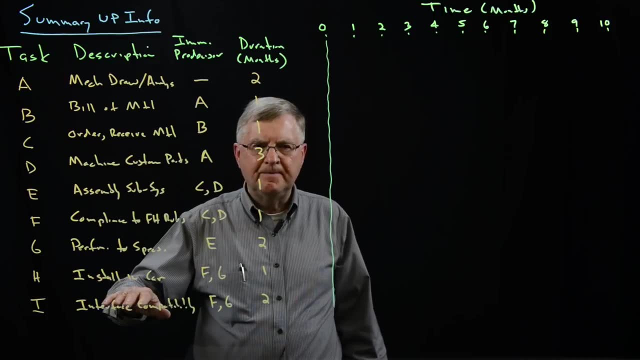 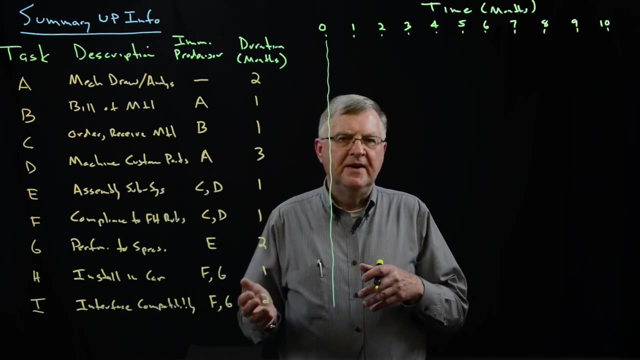 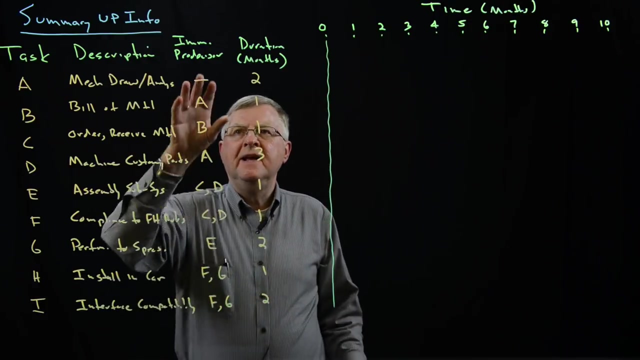 and testing the subsystem to determine if it meets the specifications or the design intent. After that, the subsystem is installed in the car and the compatibility with the various interfaces are tested, namely the mechanical interfaces and the electrical interfaces, to make sure that the subsystem performs correctly in operation. 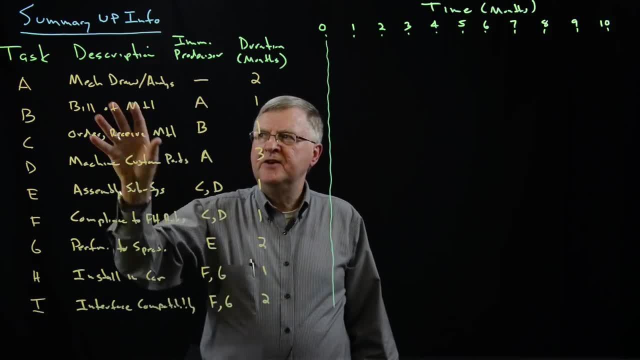 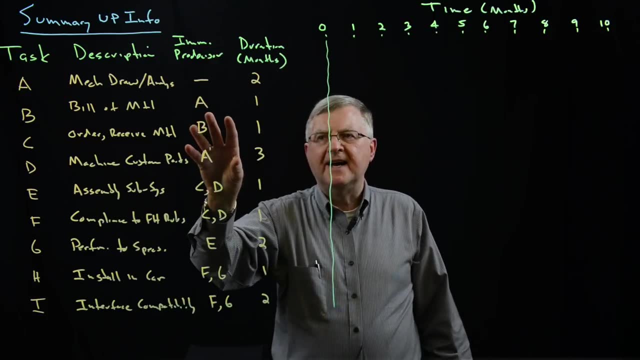 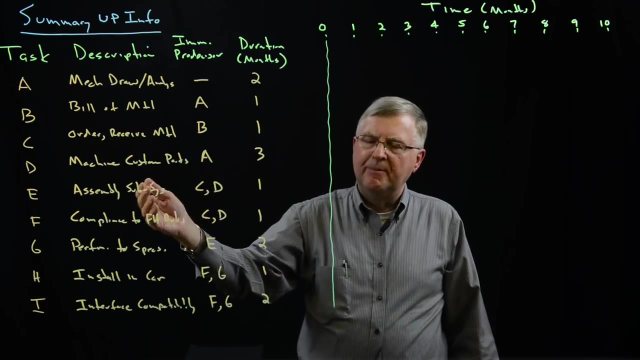 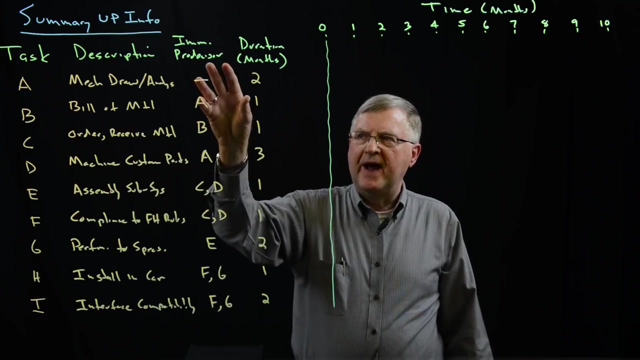 This column identifies the immediate predecessors to each of these tasks. Immediate predecessors are important because these are the tasks that generate deliverables, generate output that is used to help the following task perform its function, complete its particular tasks. Without these inputs, the particular task following: 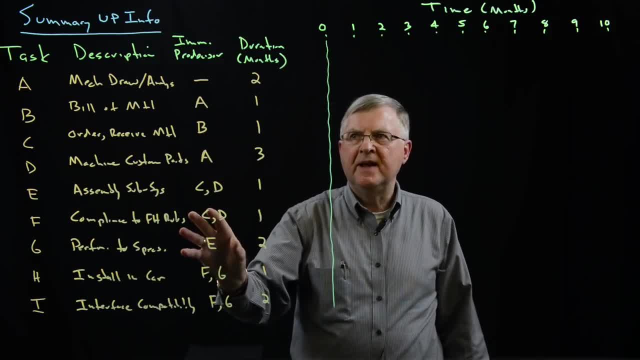 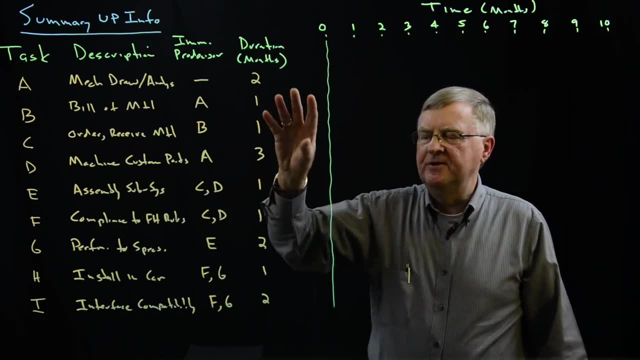 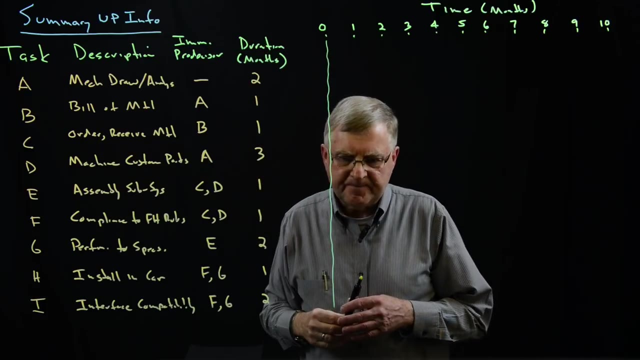 can't proceed. It needs this information. And finally, this is the duration of each of the tasks And in the work packages this duration was identified by the group performing the task. In this example, these represent months. I'm going to begin by generating the early start Gantt chart. 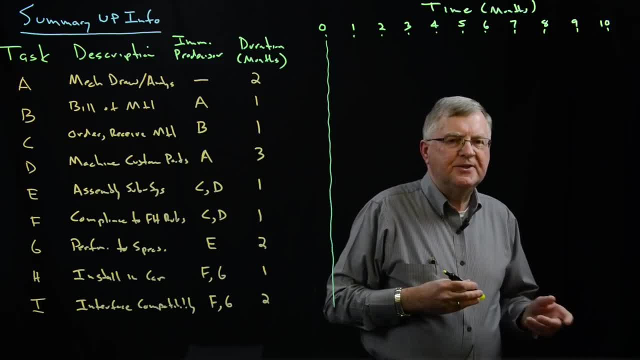 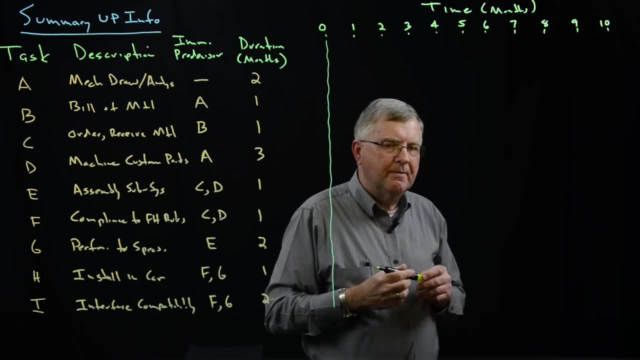 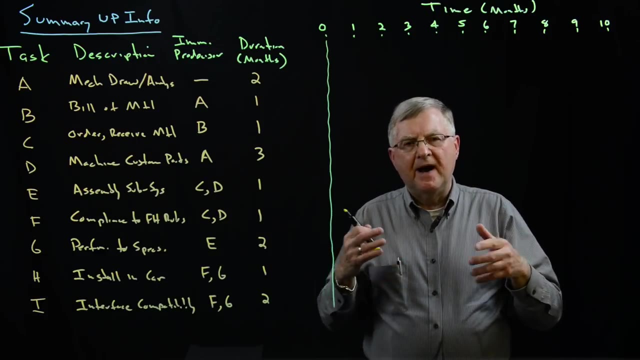 for this particular example. Now, there are various ways we could generate the schedule We could use. We could take this information And feed it into a software program like Microsoft Project and automatically generate this particular schedule. But just to help us understand how this is done, 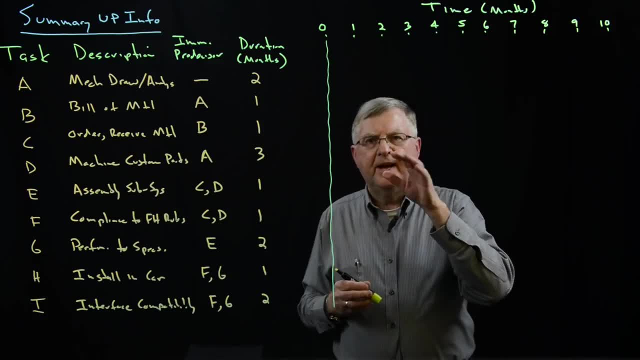 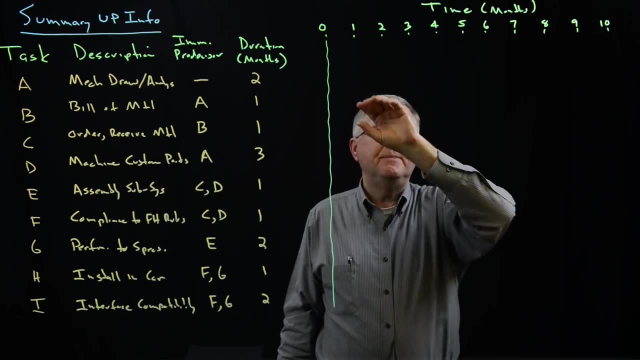 and what's going on. I'm going to generate this mechanically with a Gantt chart. A Gantt chart is a list of the activities and when they're performed in time, Across the top. here these are months, from 0 to 10 months. 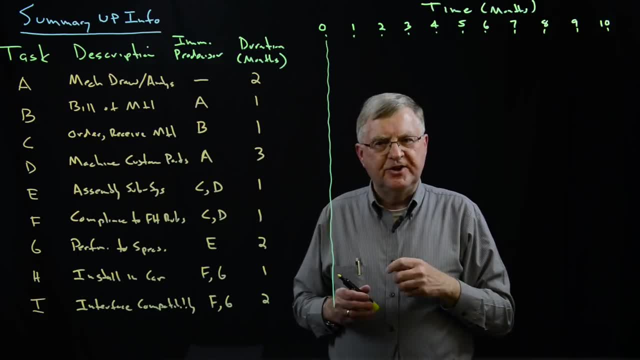 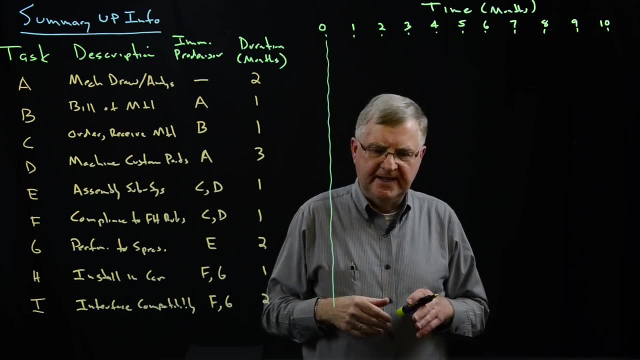 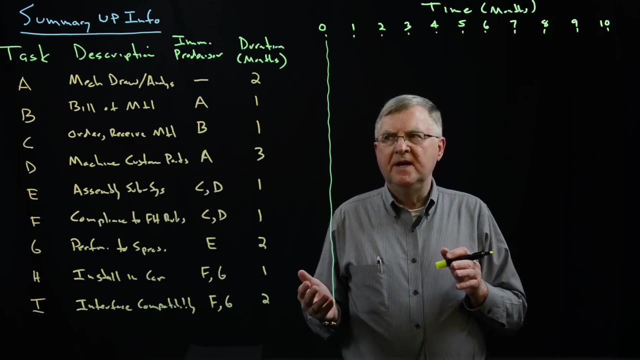 I'm going to begin by creating the early start Gantt chart. This looks at the soonest possible time that each of these activities can be initiated, the earliest time they can be completed. This is also known as the forward pass method, where I start with the first activity and work downward to the bottom activity. 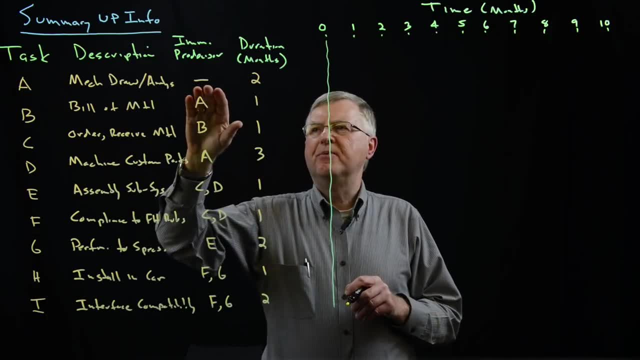 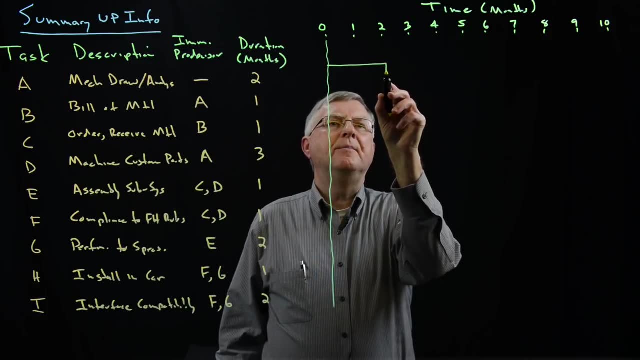 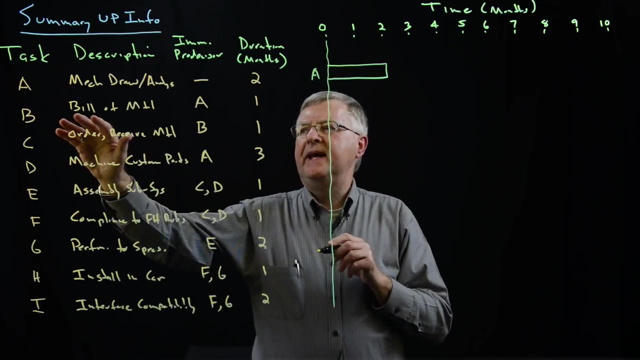 And this is how it works. Activity A has no predecessor and it has a duration of two months, So activity A can be represented by this bar in the Gantt chart. Activity B needs to be preceded by activity A and it's one month in duration. 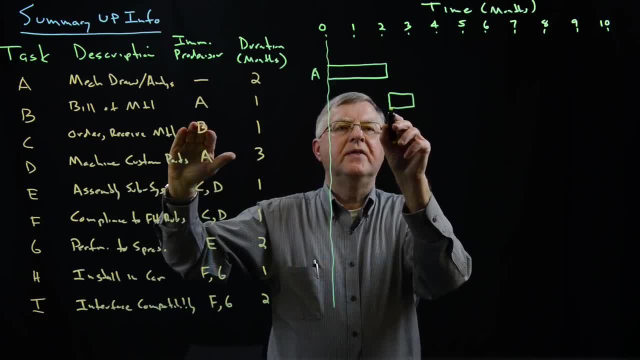 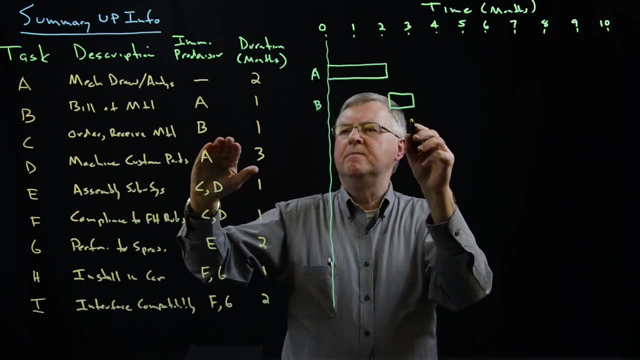 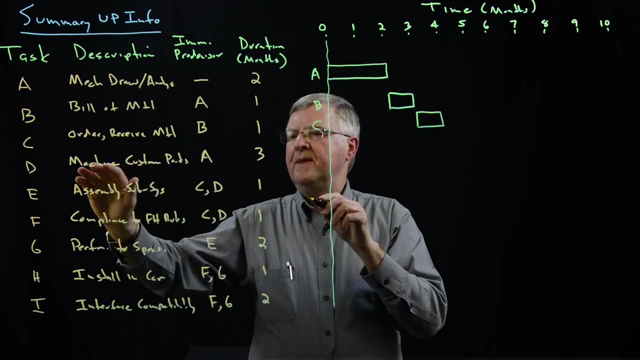 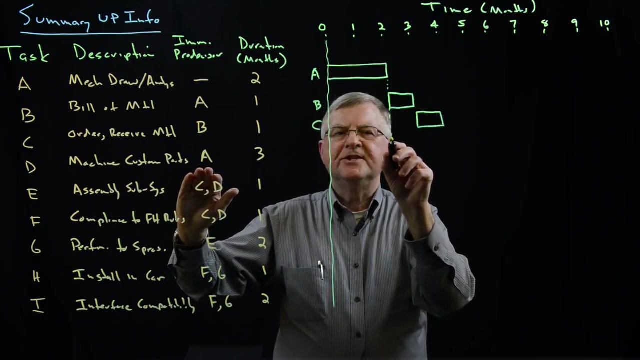 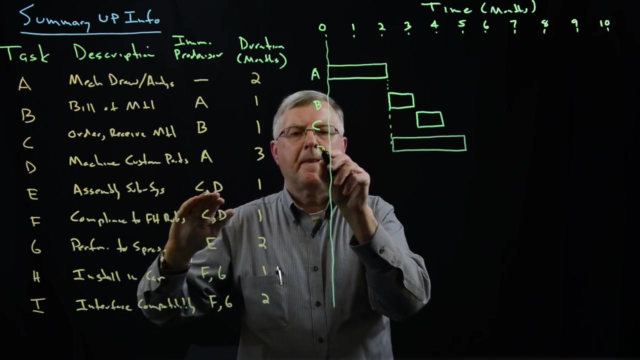 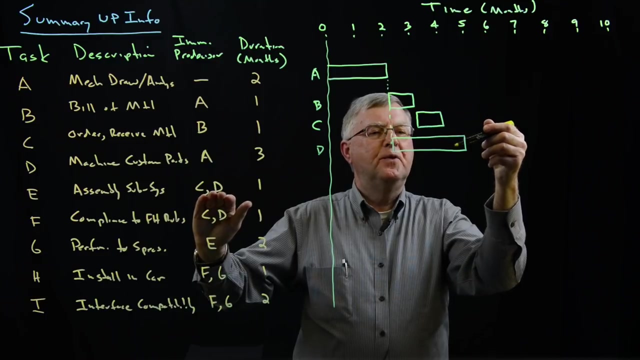 It can be depicted like this: Activity C needs to be preceded by B and it's one month in duration. Activity D is preceded by A and it's three months in duration. Activity E is preceded by C and D, but C finishes before D. 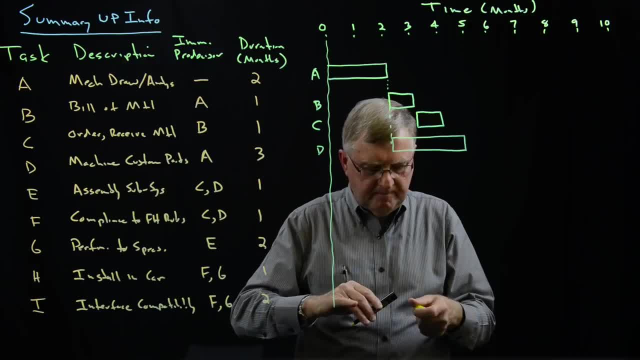 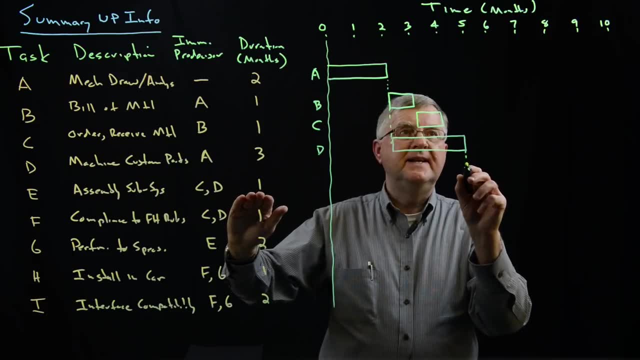 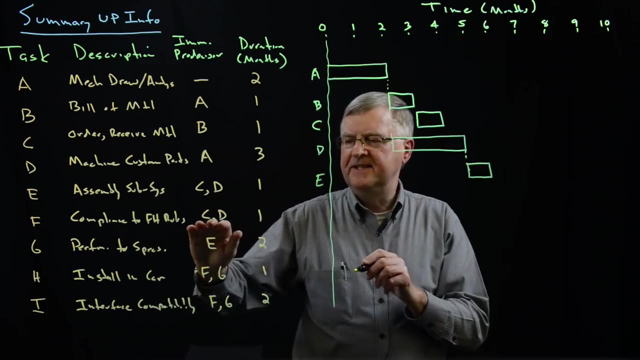 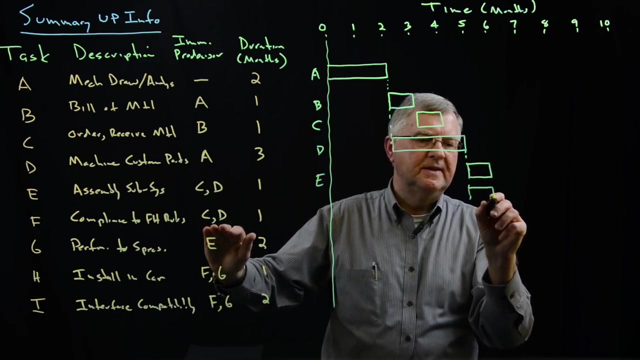 Therefore, D is the controlling item And E can't be started until E is completed and it's depicted by this. F is the same category. It needs to be preceded by C and D. It's one month in duration. It's represented by that bar. 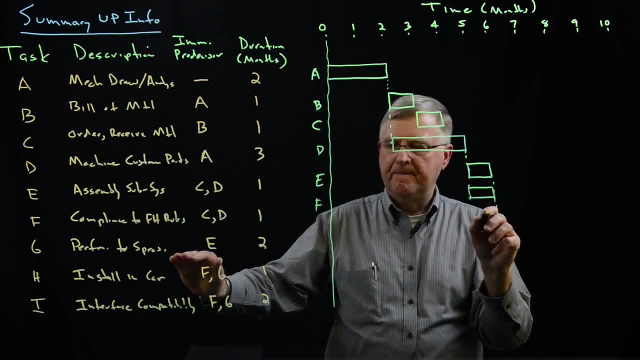 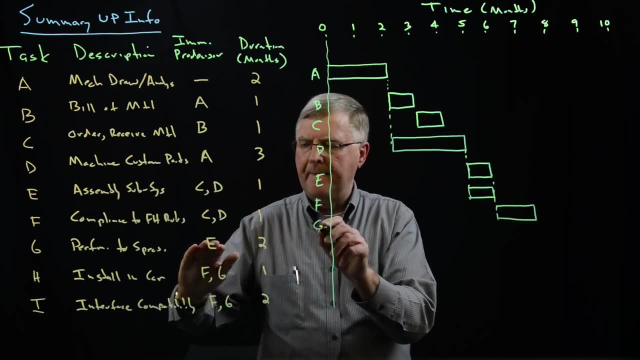 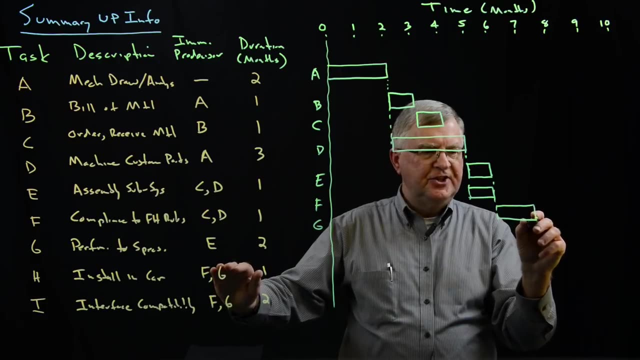 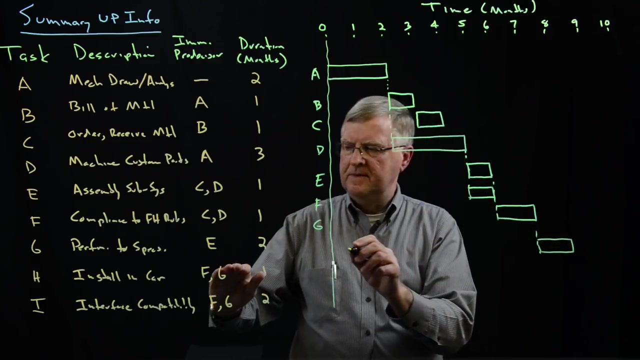 G is preceded by E …. …. … And H is preceded by both F and G. Against, G is the controller here because it's finishing last… And finally, activity I is preceded by F and G and it extends out … …. 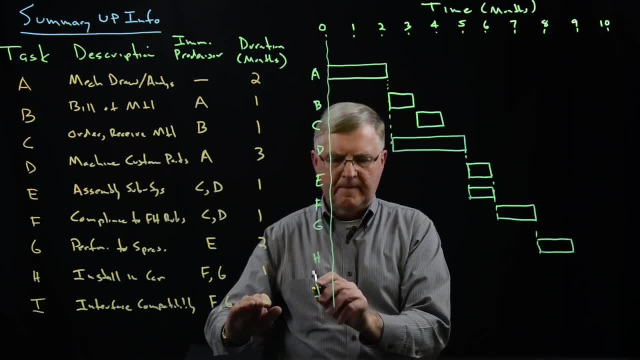 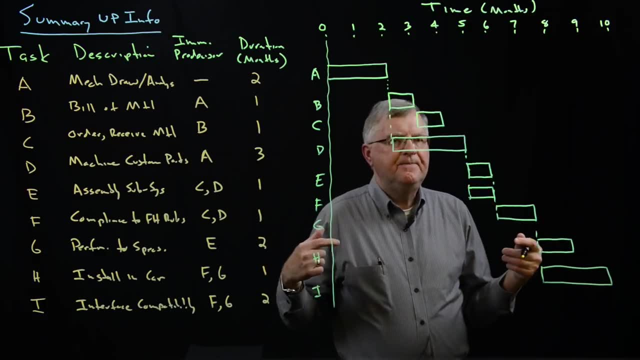 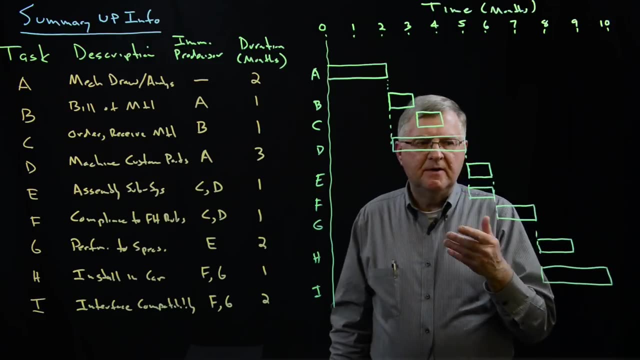 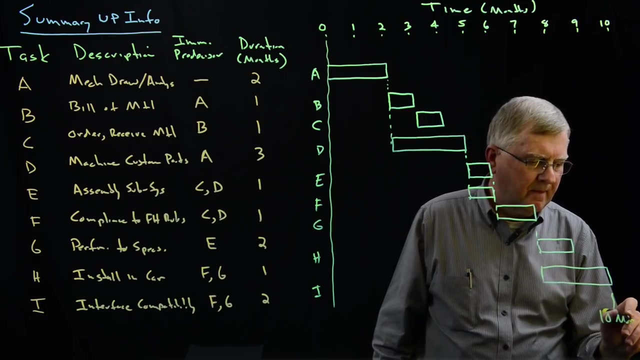 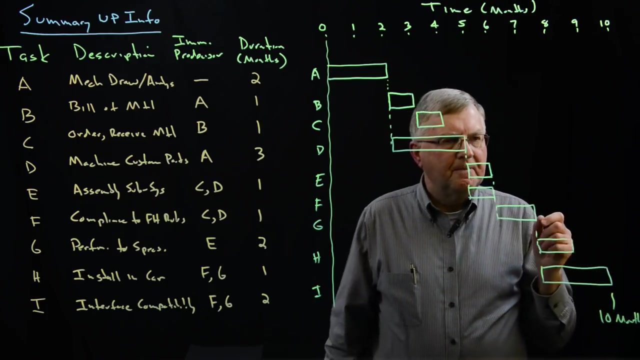 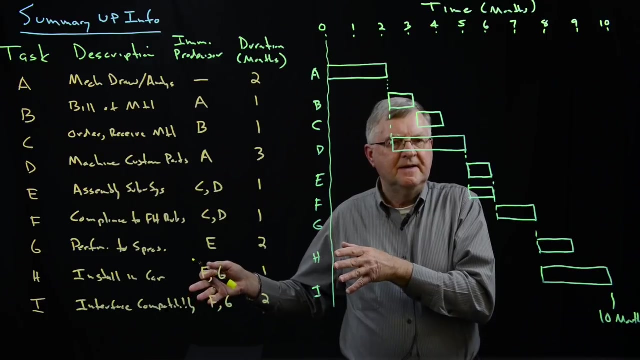 … … … … …. thusly so, we've completed the forward past analysis of our project. there's several things that we know immediately from this diagram. we know that the project is ten months in duration because this arrangement extends out ten months. so if we want to incorporate this particular subsystem in our car, we have 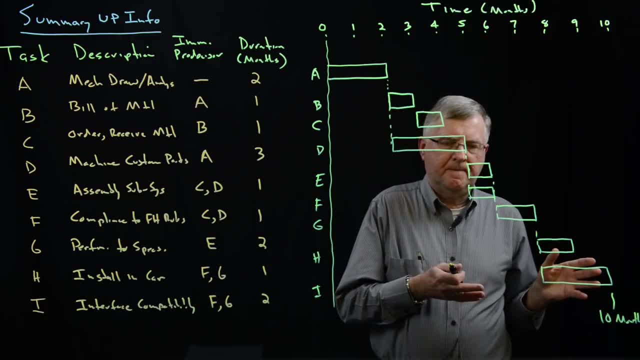 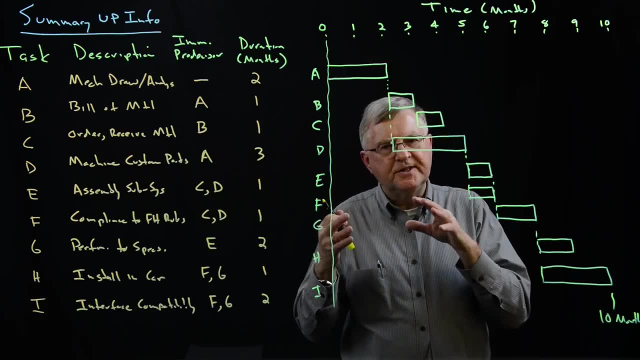 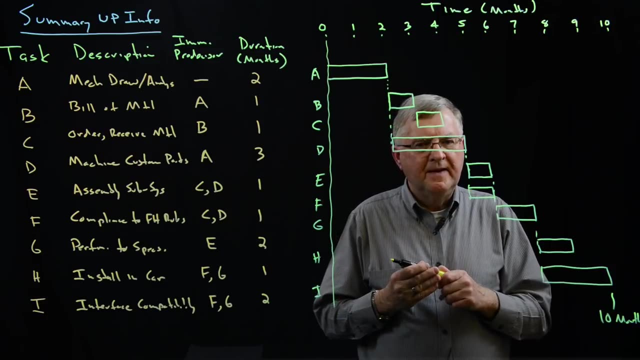 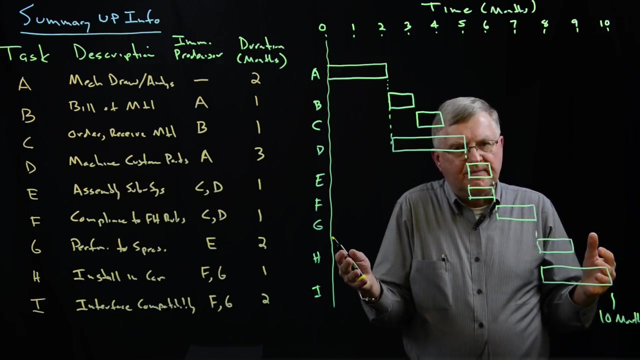 to make sure we begin the activity ten months out. if we don't have ten months, then perhaps we need to reduce the features and functionality of this subsystem to compress the schedule so we can finish it in the time allowed. this is how secondary goals and objectives are generated by a team. we would like to do something, but 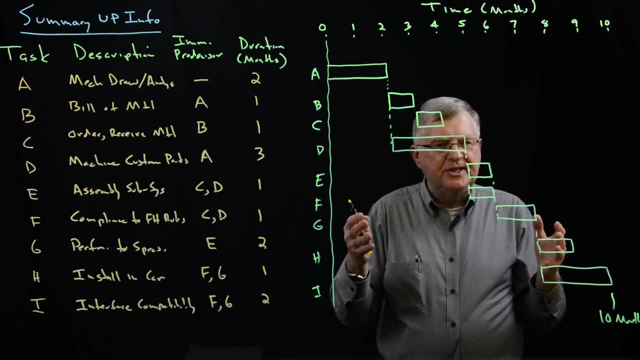 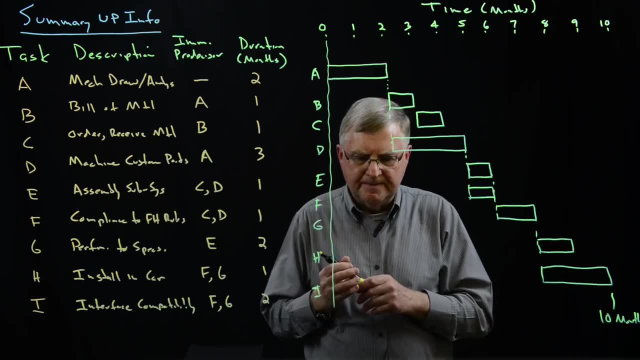 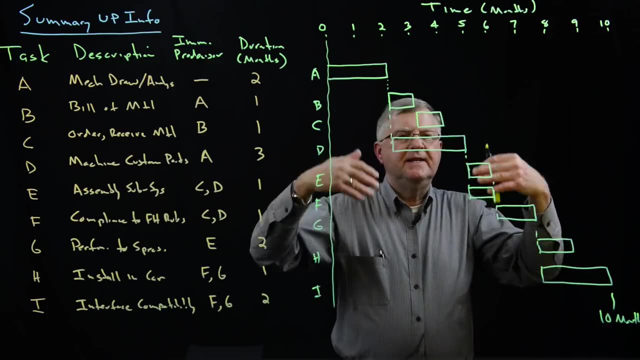 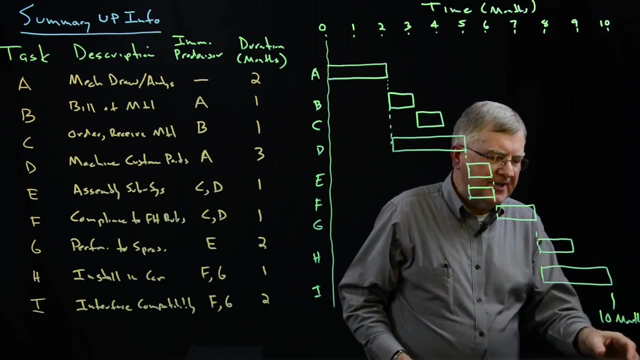 we don't have enough time to complete it. so for this year, we reduce the scope and we complete introduction of this new feature later on in the following year. now this indicates the amount of time that's required to take to complete the project. we'd also like to know about schedule flexibility. 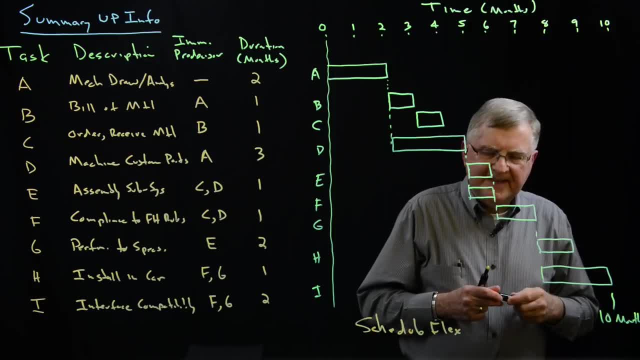 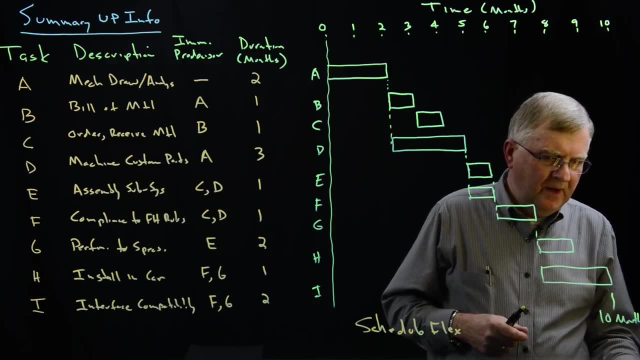 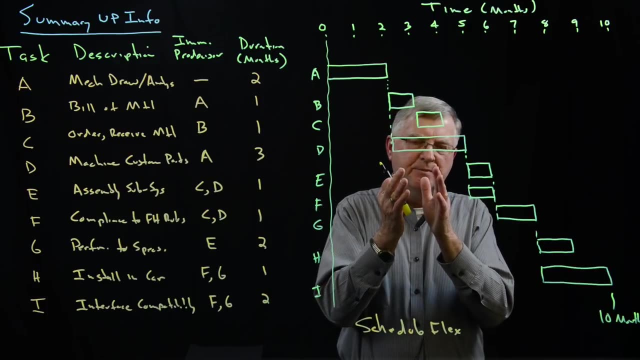 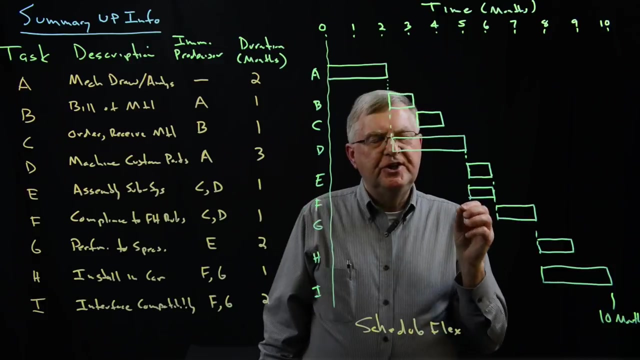 this arrangement of early start times does us and get, doesn't give us that information. so we have to do something else. we have to do a backward pass analysis to determine the range of acceptable times that each task or activity can proceed. The backward pass is just like the forward pass analysis, except we start with the very 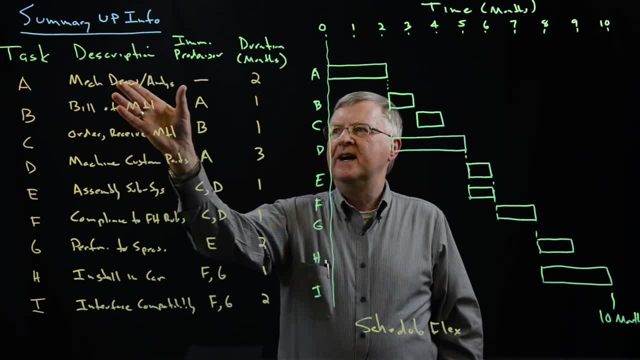 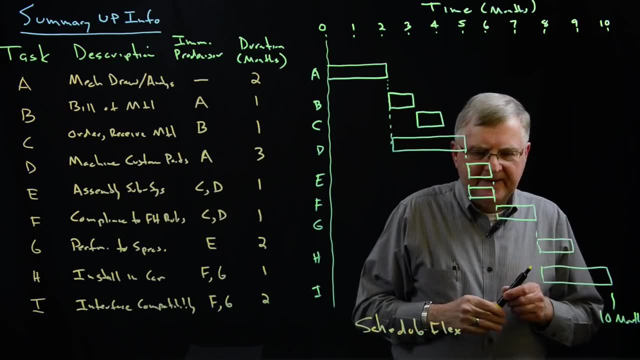 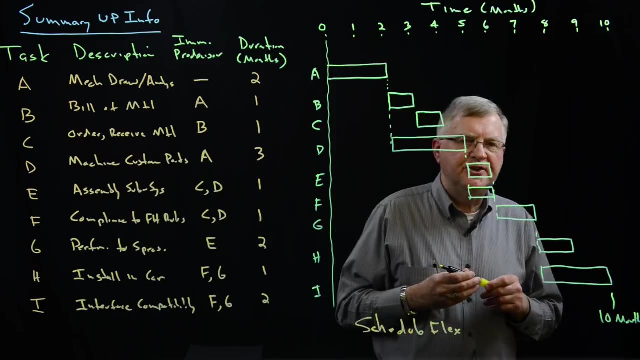 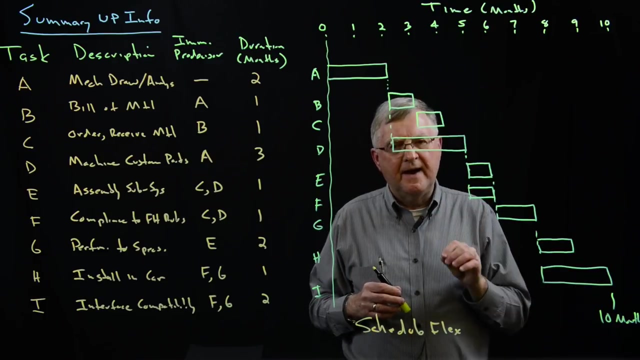 last task and we move backwards until we go ahead and complete the analysis to the very first particular item. Now in the formula hybrid rules in Appendix K there's an example showing how to do or how to perform a backward pass analysis. I'm not going to duplicate that here right now. 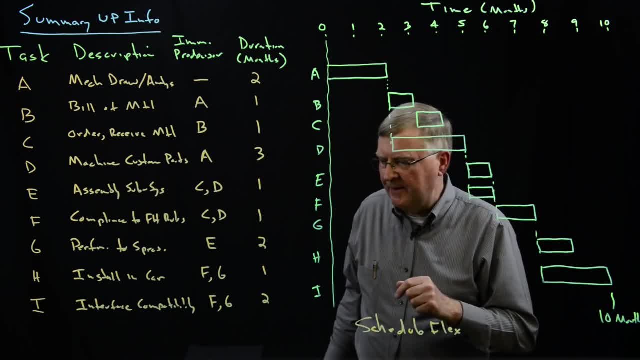 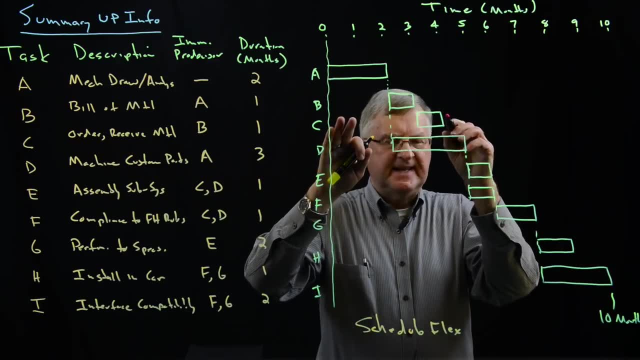 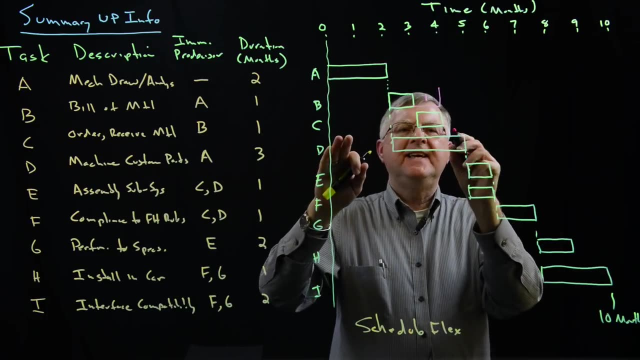 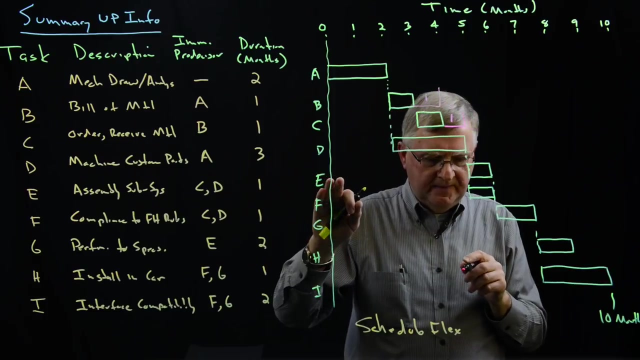 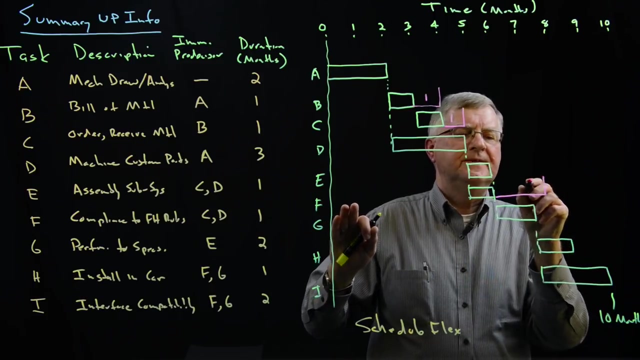 What I will do is put the results in of the backward pass, And the results are as follows: Activity B can extend out 1. More month. Activity C can extend out in duration 1 more month. Activity F can extend out 2 more months. 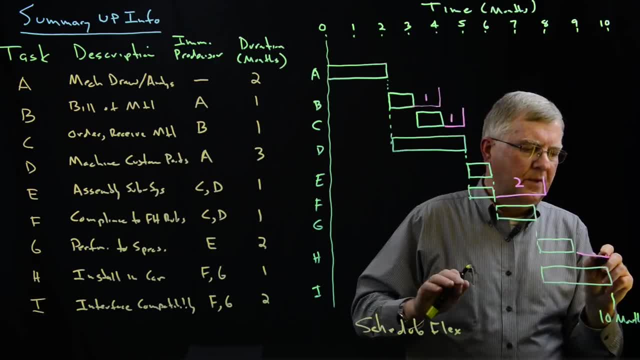 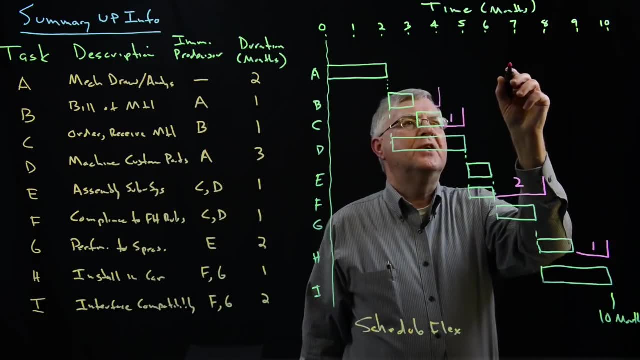 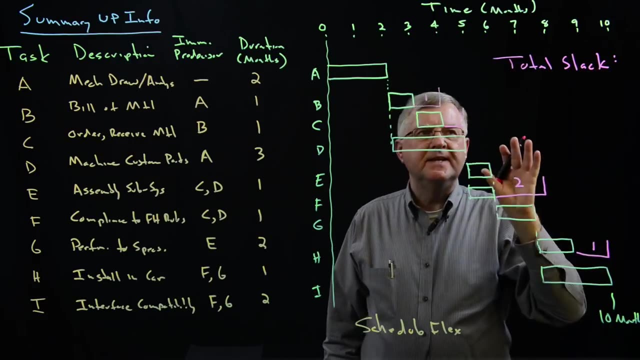 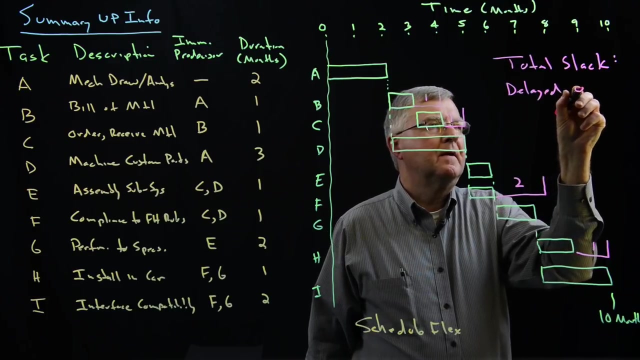 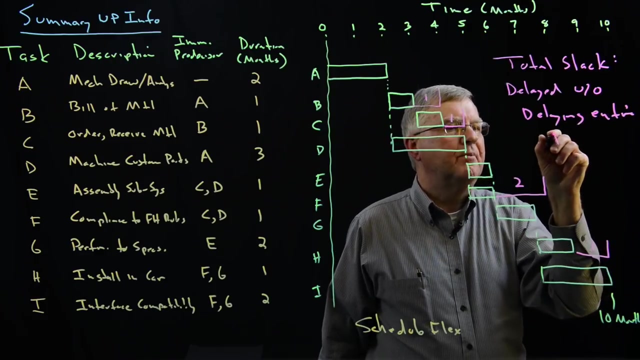 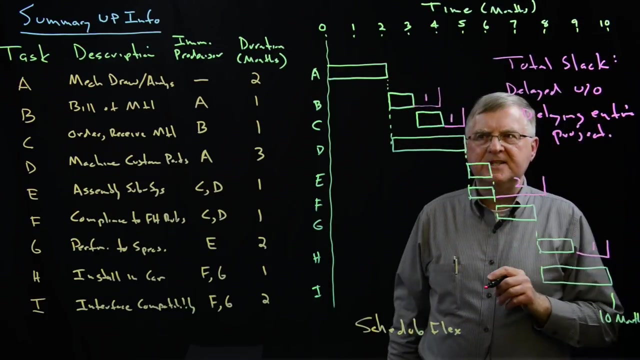 And activity H can extend out 1 more month. Now, what I've shown in red here is called total, That's the interval slack. This is the amount of time these activities can be delayed without delaying the entire project. We have flexibility, then, in these 4 activities. 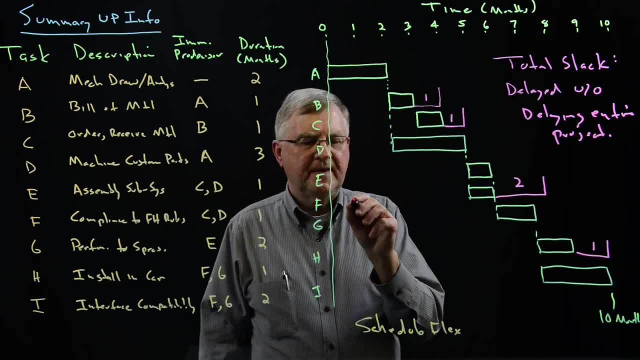 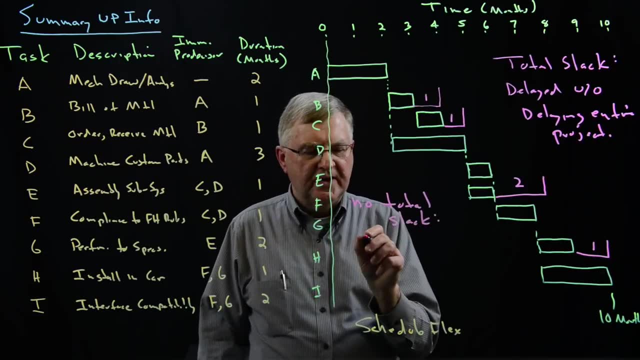 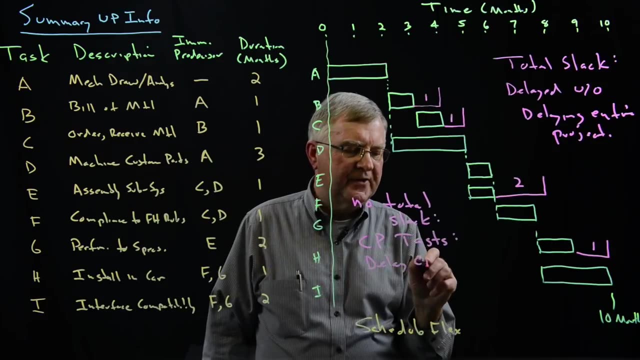 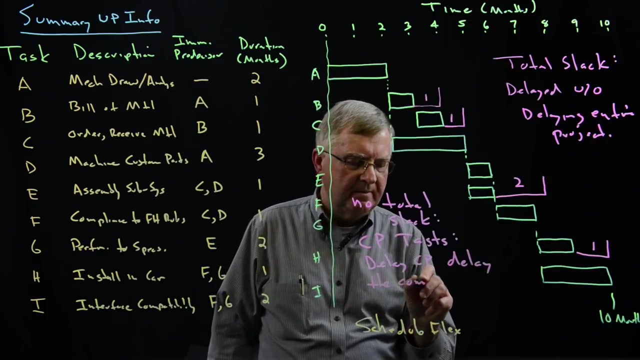 The other 5 activities are defined here In the model. we're going to see how to add them. The five activities have no total slack. As a result, they're called the critical path tasks or activities. Delay in the critical path tasks will delay the completion of the entire project. 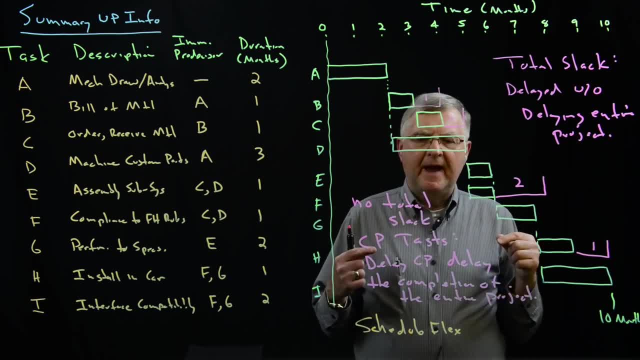 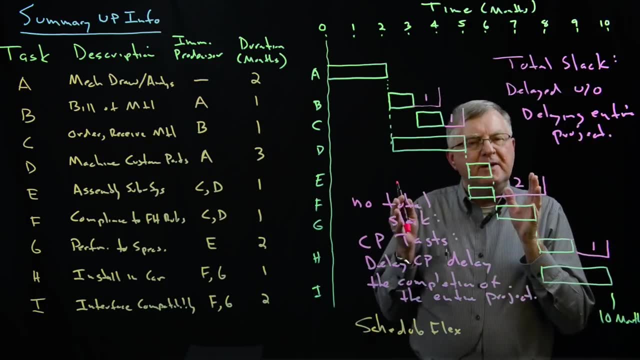 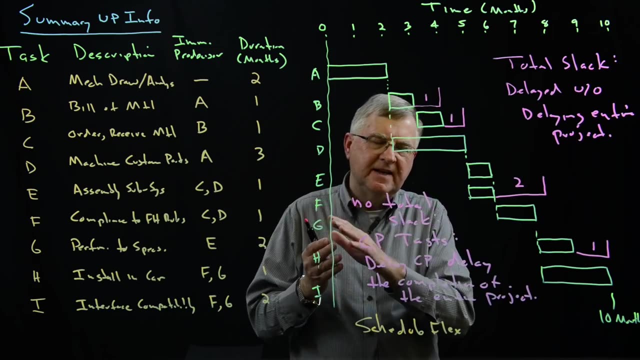 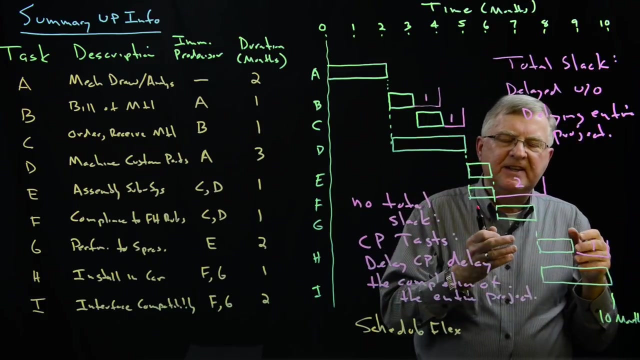 Therefore, as project manager, I want to identify the critical path activities, because those are the activities that I'm going to be managing very carefully to prevent delays in those activities from impacting the entire project. I'm going to be managing to the activities that have total slack, because they allow me to move resources around the project.